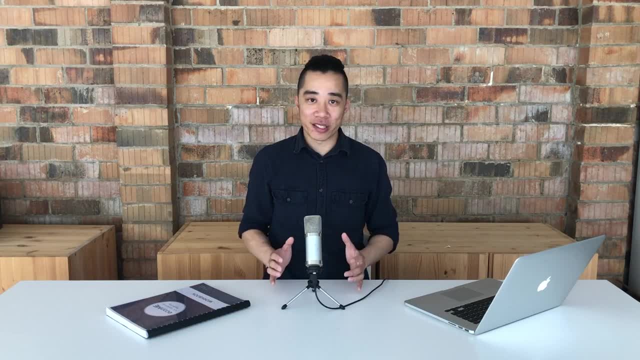 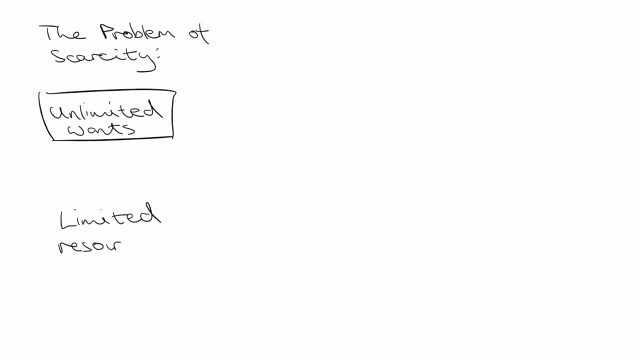 build on these concepts later in the course. All right, let's start off with the definition. At the start of the economics course, we'll learn of the problem of scarcity. We have unlimited wants but only limited resources to satisfy them. Therefore, we must make the choices of: 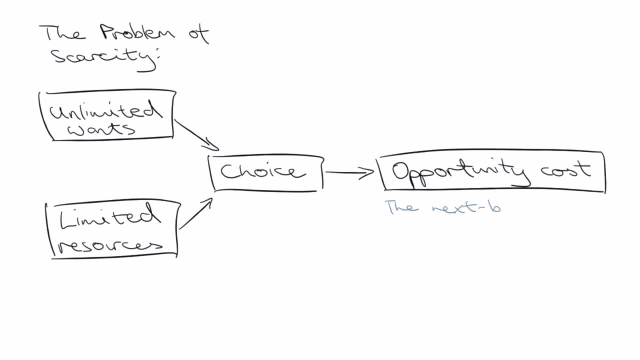 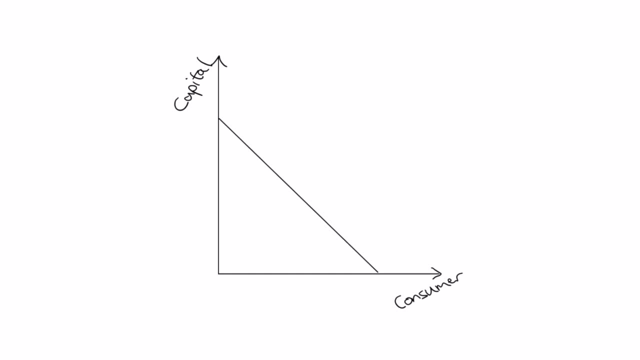 which wants to satisfy and which wants to sacrifice. The next best alternative that is foregone for satisfying one want is the opportunity cost. The production possibility frontier, or PPF, is a graphical representation of opportunity cost. It is also known as the production possibility curve or PPC. It is a model that shows the combination of two products. 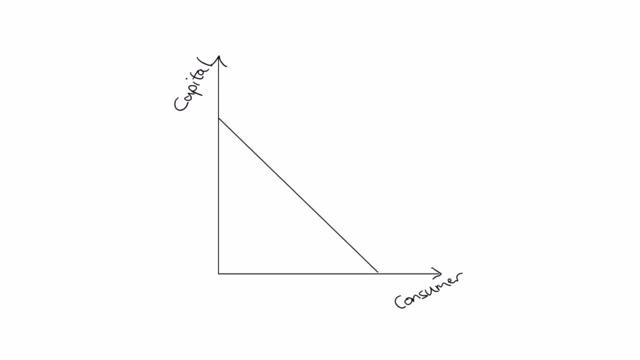 that an economy can produce if it used all of its resources to their full capacity. To draw a simple PPF, we must make the following assumptions: The economy is only producing two products, like apples versus oranges. The state of technology and the quantity of resources are fixed. 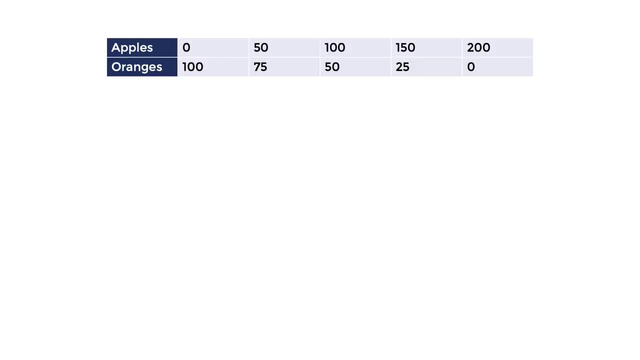 And thirdly, all resources must be fully employed. Now let's draw a PPF using this production possibility schedule, which is what we call a table of data in economics. Let's start with labeling our axes and plotting the points from the schedule. Here's a hint, If you know it's 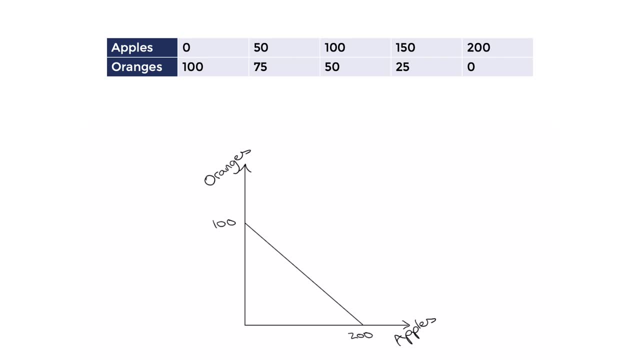 a straight line. you could just plot the ends and then join them. The schedule and curve shows the combination of apples and oranges that the economy could produce if it used all of its resources to their full capacity. As you can see, if we used all of our resources for apples, we would be on this end of the PPF, making zero oranges. 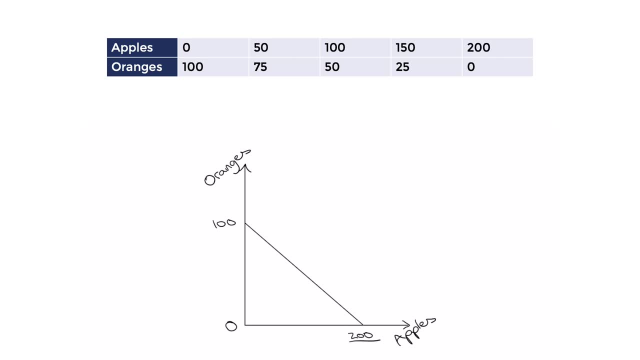 and 200 apples. If we used all of our resources on oranges, we would make 100 oranges and zero apples. If we split our resources between the two, we'll be operating on the line and making combinations like 100 apples and 50 oranges. Now what does this model have to? 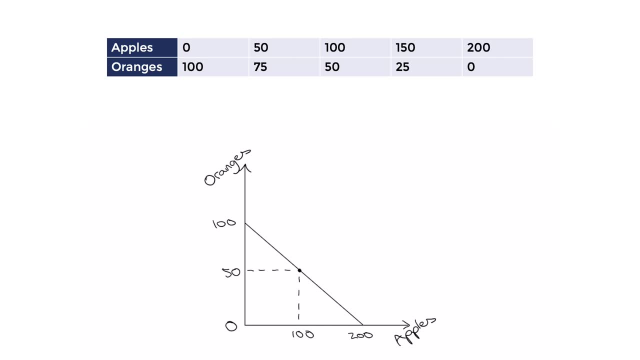 do with opportunity cost. Well, this model is built on the concept of choice. Because of scarcity, any combination we choose will involve sacrificing the alternative one. Let's use our apples and oranges example to show how to calculate opportunity cost. Let's start at the extreme and 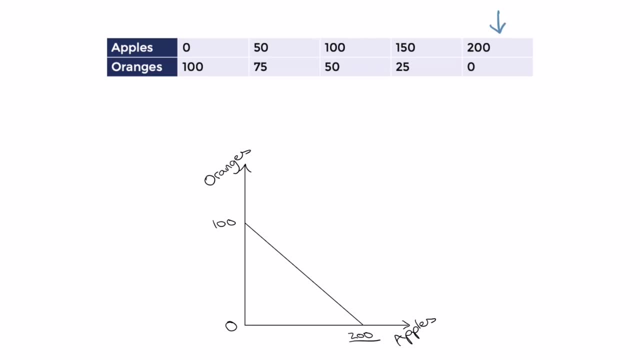 put all of our resources into producing apples, We'd have 200 apples and zero oranges. Now let's say we want to produce 25 oranges. By moving from zero oranges to 25, we'd be reducing our apples by 50.. This shows that to produce 25 oranges we would have to give up 50 apples. This 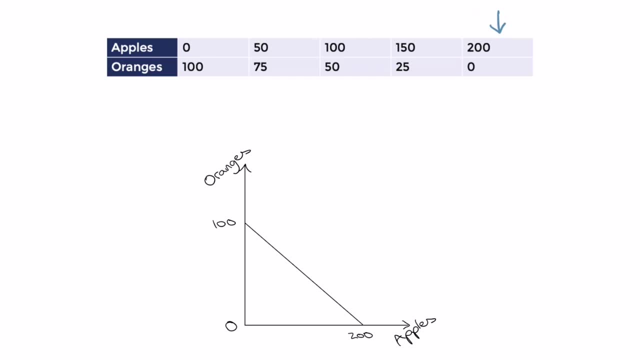 is the opportunity cost. Let's say we want even more oranges. If we increase production to 75 oranges, that would bring the total opportunity cost up to 150 apples that we had to sacrifice to make these 75 oranges. And if we shift all of our resources to oranges, 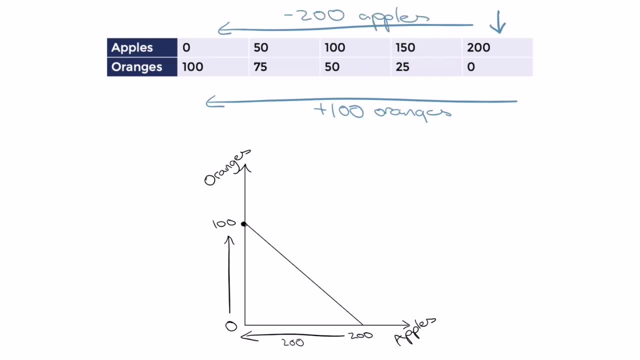 we'd make 100 oranges and the opportunity cost is 200 apples, because that's what we've given up in total. One more helpful skill to learn is figuring out the per-unit opportunity cost of producing each good. Let me show you how to do it. If producing 200 apples has an 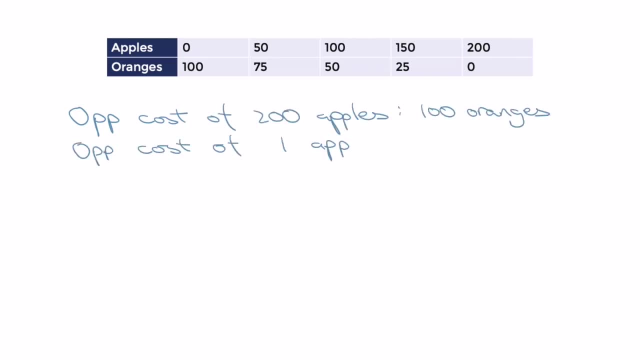 opportunity cost of 100 oranges. the opportunity cost of producing each apple would be 100 oranges divided by 200.. Half an orange is the opportunity cost for each apple produced. On the other hand, the opportunity cost of 100 oranges is 200 apples, so the opportunity cost of each orange is 200. 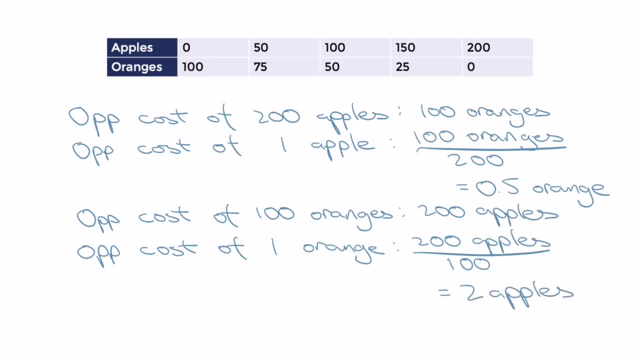 apples divided by 100. Two apples are sacrificed for each orange produced. This would mean that if we look at our orange production as a whole, we would have 100 oranges. but if we per unit opportunity cost is called marginal rate of substitution or MRS- The MRS can also be- 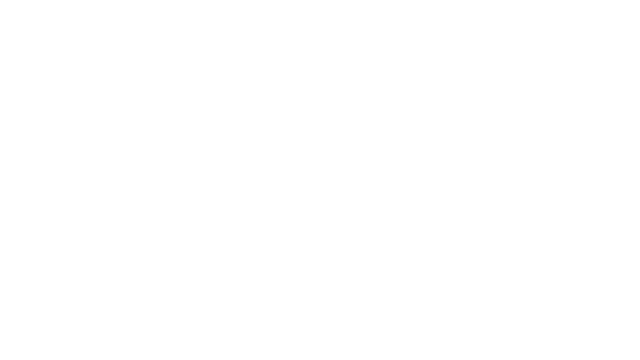 observed in the gradient of this PPF, and so we've covered how to draw the PPF and calculate opportunity costs. I'm now going to explore some factors that could change the PPF. Let's look back at the assumptions that we fixed earlier. Let's see what happens if we change this middle assumption. 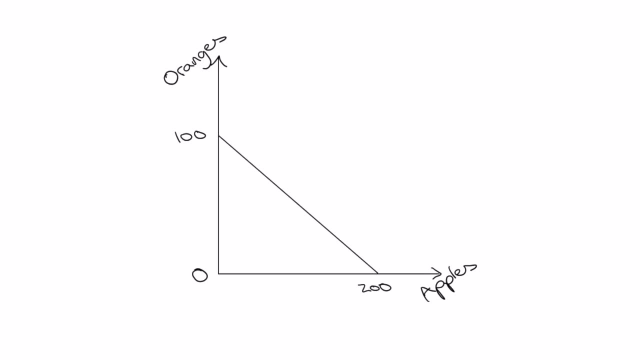 about technology and productivity. Improvements in technology or productivity would mean that this economy could increase its production. with the current resources, This would mean that the economy has increased its productive capacity and the PPF would shift outwards. If the technology or productivity improvement applies only to apple production, it would look like this: We would 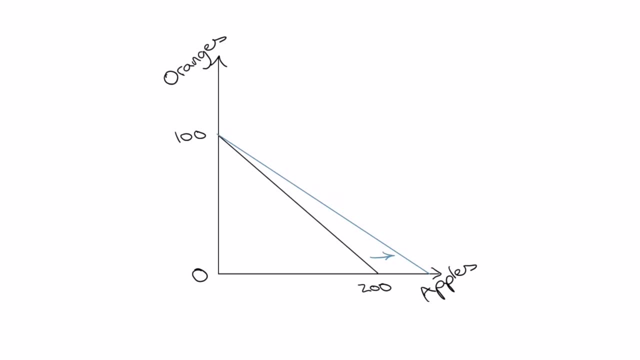 shift the line outwards only from the apple side. An example would be if we introduced an apple specific fertilizer or if workers received training and gained expertise for apple farming. On the other hand, if the improvement applies only to orange production, the line would shift outwards. 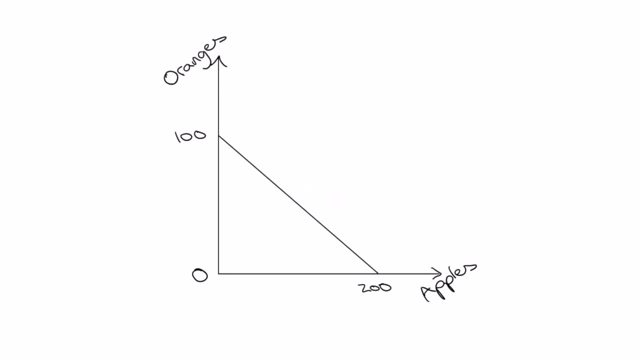 from the orange side. If the improvement applies to both apples and oranges, the whole line would shift outwards. An example would be gaining a tractor that can be used for harvesting both apples and oranges more efficiently, because this means we can make more of both. The discovery of new resources would have a similar. 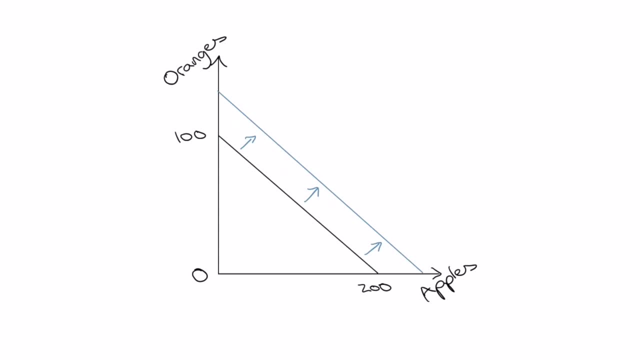 effect. They would shift the PPF outwards depending on the applicability of these resources. For example, gaining arable land to grow either apples or oranges would shift the PPF outwards because, again, we can produce more of both. Another assumption we could relax is that all resources are fully. 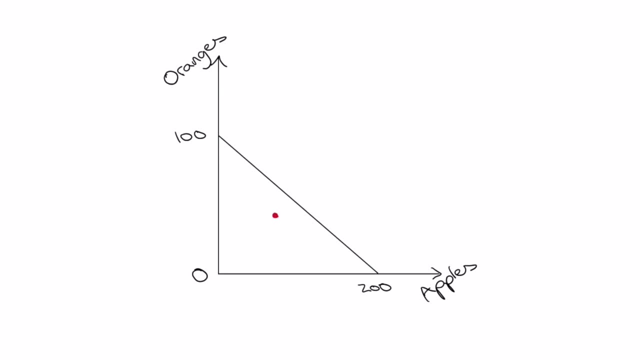 employed. If we're experiencing unemployment of resources, the economy would be operating inside red combination. It doesn't usually shift the PPF because the potential for high production is still there. We're just producing a smaller combination because we're not using our land labor capital. 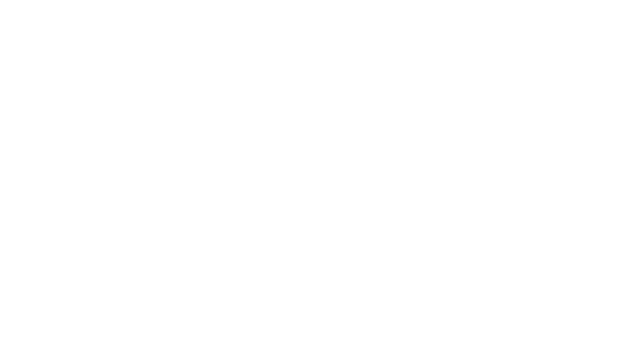 enterprise to this full potential. Now there's one more assumption that we've been working with. up to this point, We've been assuming that the PPF is a straight line. This means that all of the economy resources are perfectly substitutable between apples and oranges, But in reality, some resources 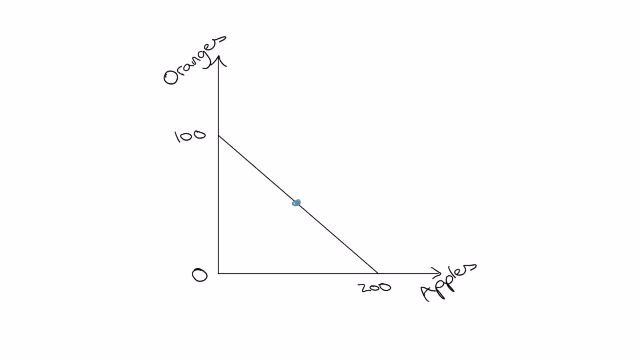 more suited to growing apples and some suited to growing oranges. So as we move to the extremes, we will lose some productive capacity. For example, if we decide to only make oranges, some apple-specific resources will be lost, causing us to lose productive capacity at this. 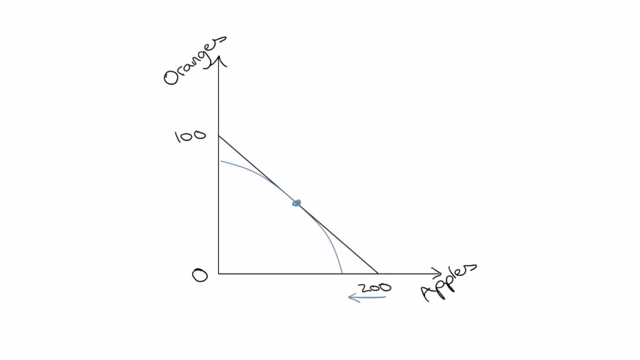 extreme And same on the other side. we will lose some apple-specific resources if we only make apples. This leaves us with this concave-shaped PPF. Okay, one last concept to explore. There are certain choices that we make with the PPF that can have future implications. Consider this PPF. 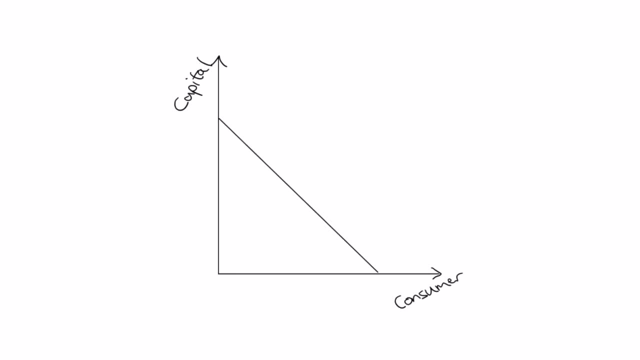 where we must choose between consumer goods and capital goods. Consumer goods are items for satisfying current or immediate wants, like a holiday. On the other hand, capital goods are items that can increase efficiency and therefore help to satisfy future wants and needs instead of today's, like machinery or education. What would happen if we focused more? 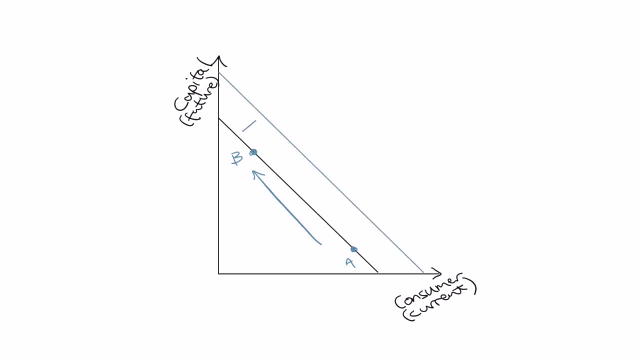 on producing capital goods. It would lead to increased productive capacity in the long run, allowing us to be able to produce more of both consumer and capital goods. The PPF would shift outwards, but the opportunity cost is the ability to satisfy current consumer wants. 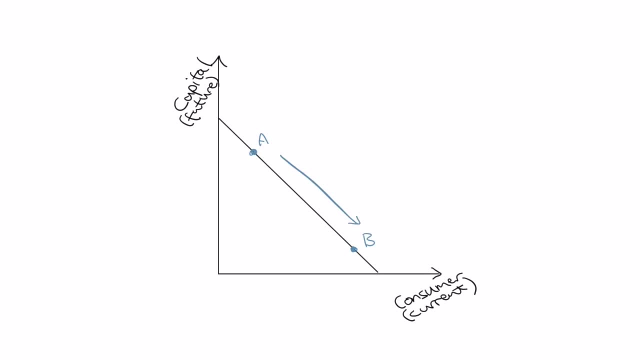 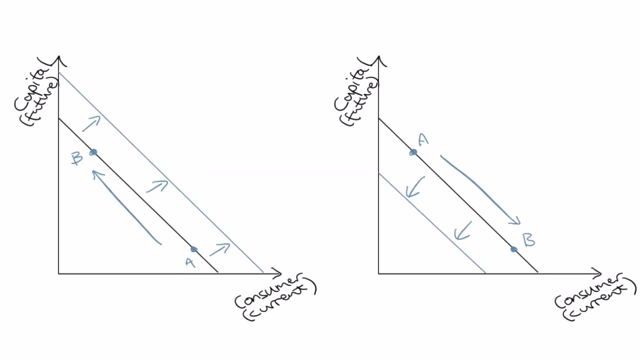 What if we went the other way and focused only on producing consumer goods? We'd be happy today, but in the long run we would run out of resources and be able to produce less of both. This model highlights the importance of investing into new technology and sustainability, even if it means